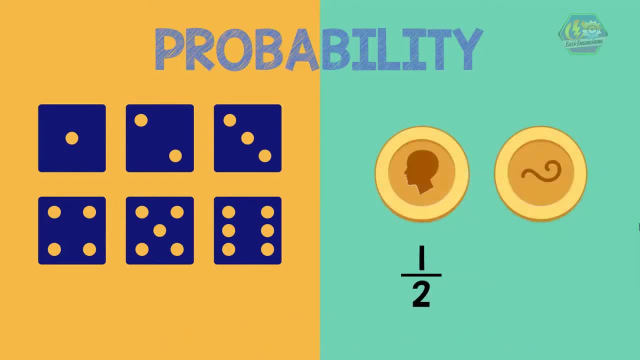 That means that probability of coin landing heads is one half and the probability of coin landing tails is also one half. Also, when we roll a single dice, there are six possible outcomes we can get, So this means that the probability of any one of them is 1 over 6.. 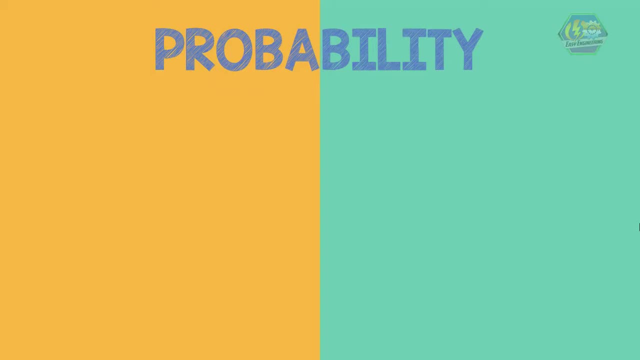 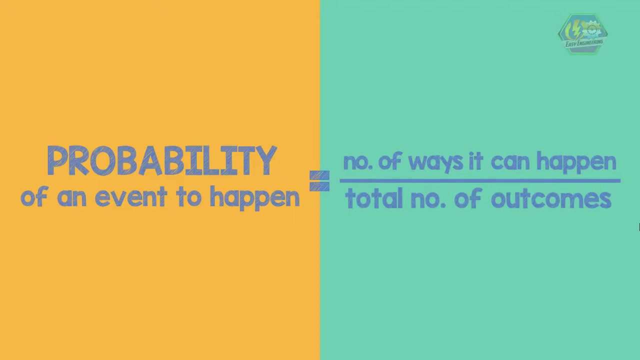 So, in general, in order to know the probability of an event to happen, we just need to divide the number of ways it can happen by the total number of times the total number of outcomes. Let's try to visualize it by using the probability line. 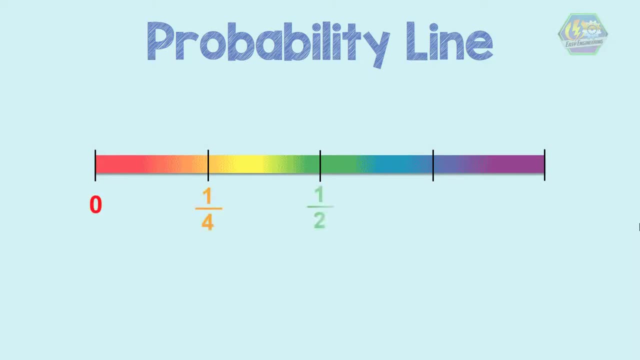 Probability line is just like a number line that goes from 0 to 1.. A probability of 0 means that the event is impossible to happen, And a probability of 1 means that the event is certain to happen, And a probability of 1- half means that there is an even chance that the event will happen. 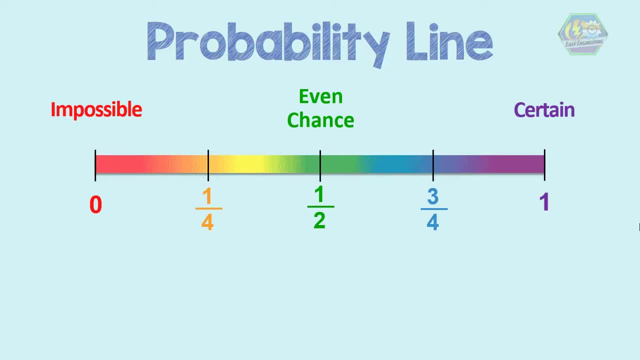 or not. The probability less than 1 half means that event is unlikely to happen, And the probability greater than 1 half means that event is more likely to happen. We can also use percentage to represent the probability. line 0 is simply 0%. 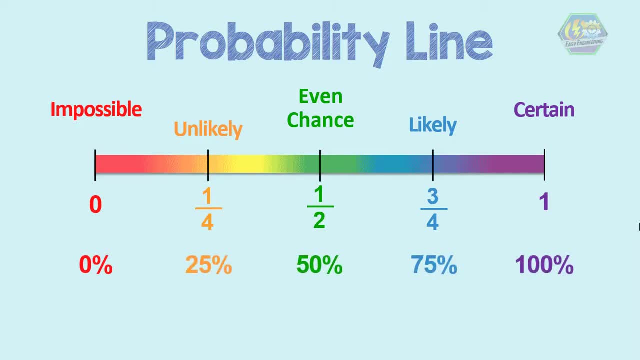 1 half is 50% And 1 is 100% In the case of tossing a coin. since there are 2 possibilities, then we have to divide the probability by 2.. So 1 divided by 2 is 1 half or 50%. 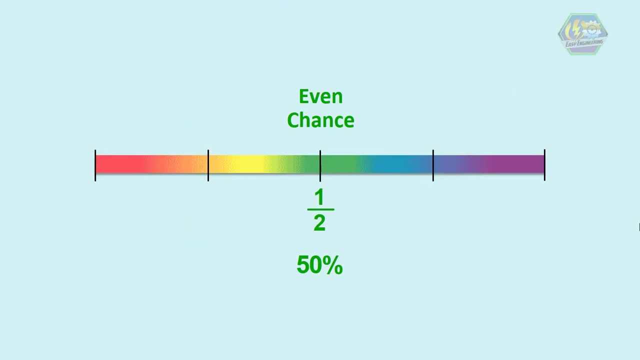 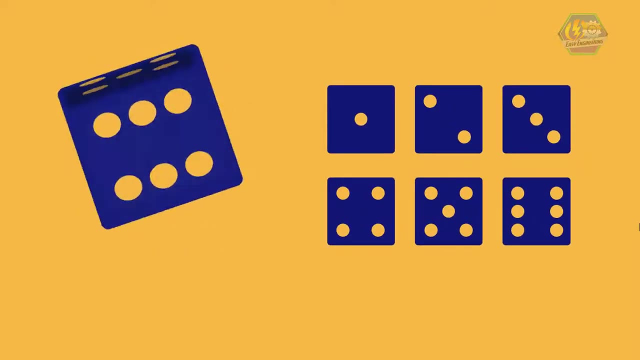 Therefore, there is an even chance that the event will happen. In the case of rolling a dice, there are 6 possibilities. 1 divided by 6 is 1 over 6, which is equivalent to 16.7%. So this means that it is unlikely to get a certain number of instance, but it is just. 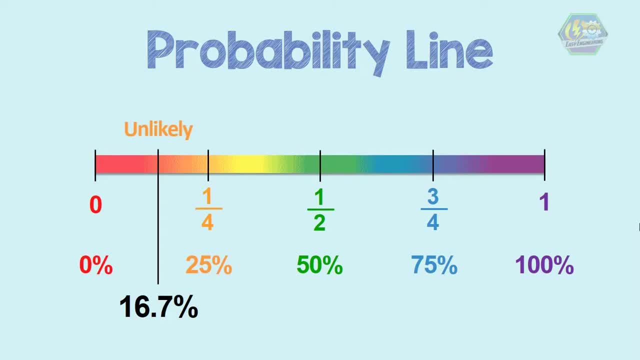 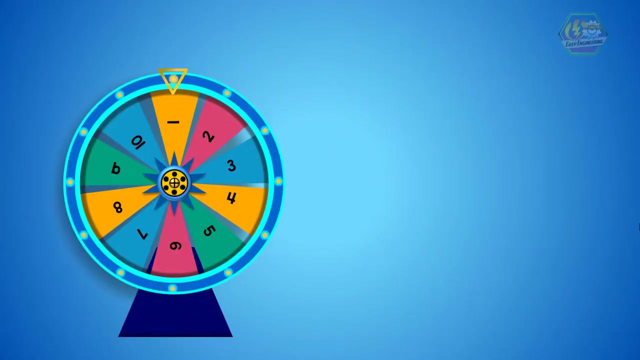 as likely as rolling any number. Now let's have some examples to further understand probability. For example, in the case of tossing a coin, What will happen? 1 divided by 2 is 1 half. What will happen? You have a random number wheel that has a number from 1 to 10.. 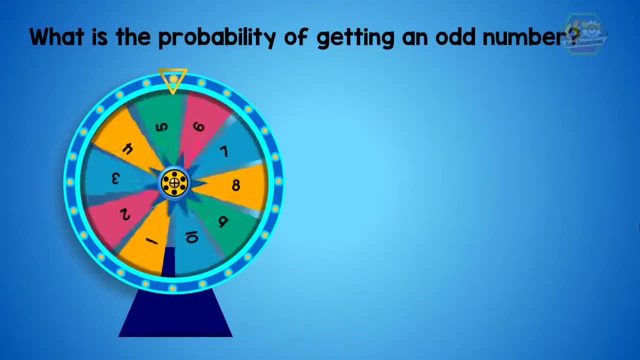 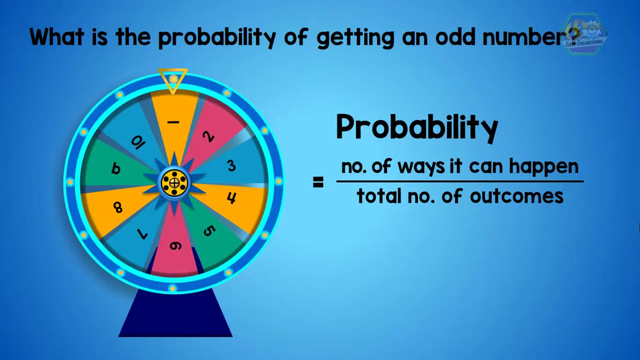 What is the probability of getting an odd number? So let's use the formula in getting the probability of an event, which is the number of ways it can happen divided by the total number of outcomes. There are 5 odd numbers in the wheel, which are the numbers 1, 3, 5, 7, 9.. 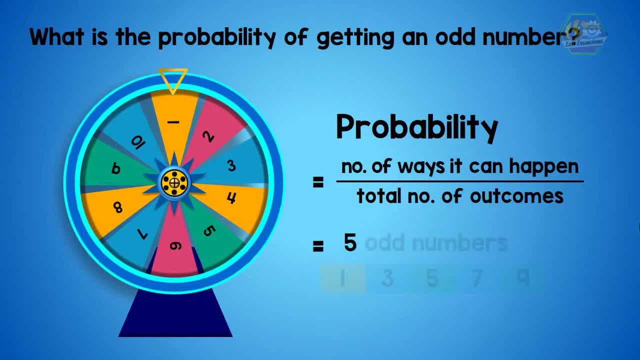 Therefore the number of ways it can happen is equal to 5.. And there are 10 numbers in the wheel, So the total number of outcome is 10.. So 5 divided by 10 is 5 over 10.. Or 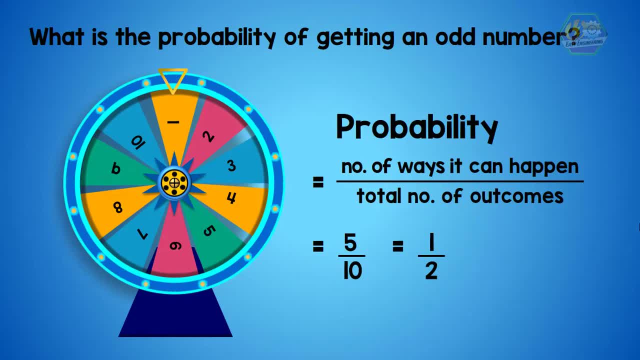 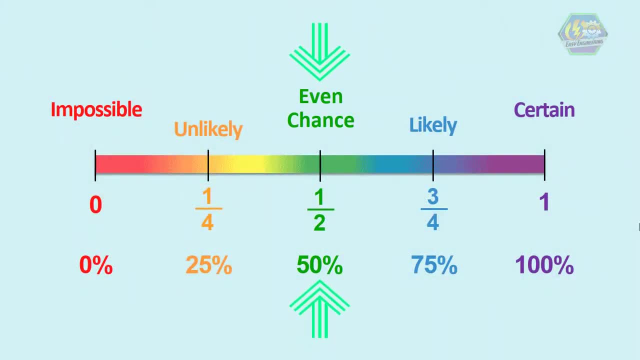 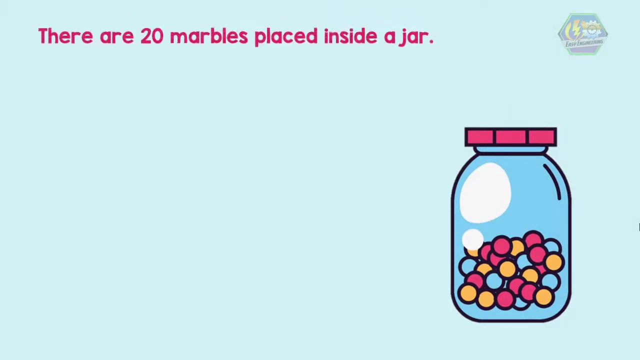 1 half. Therefore, the probability of getting an odd number is 1 half or 50%. So it's right here at the probability line. That means there is an even chance an event will happen. Okay, for another example, There are 20 marbles placed inside a jar. 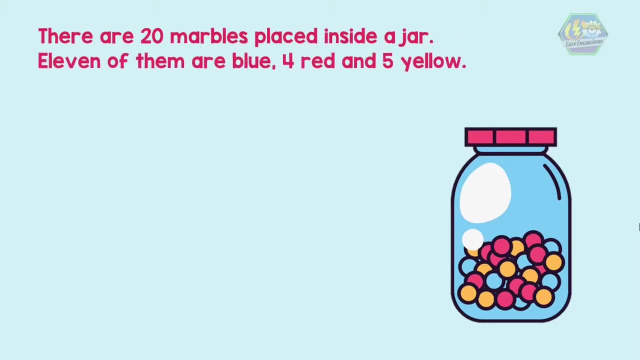 11 of it are big, 2 are blue, 4 are red And 5 are yellow. What is the probability that a red marble will be picked? So, again, let's use this formula to find the probability. There are 4 marbles. 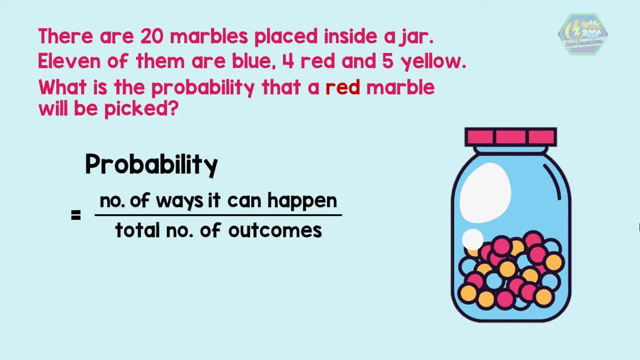 So this means that the number of ways it can happen is equal to 4.. And since there are a total of 20 marbles in the jar, So that means that the total number of outcome is 20.. 4 divided by 10 is 4.. 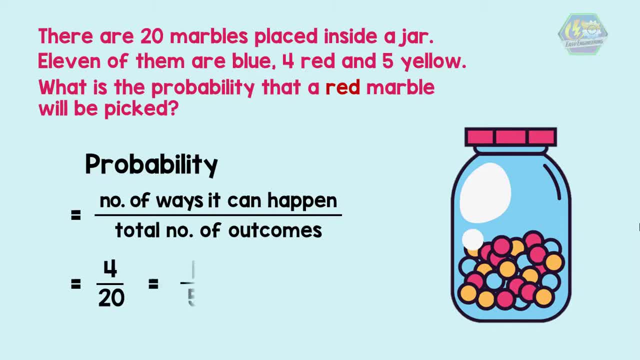 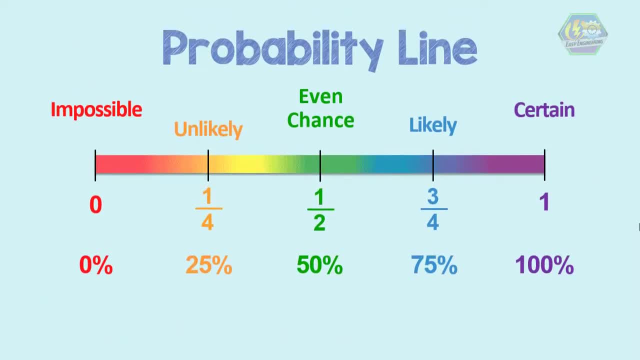 5 divided by 20 is equal to 4 over 20, or 1 fifth or 20%. So it's right here in the probability line That means it is unlikely And that makes sense, since it would be less likely to pull a red marble than the other marble.